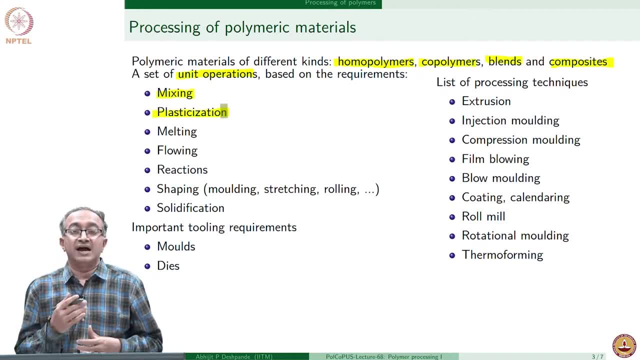 example is an example of an additive where we add the plasticizer to improve the flowability of the material or also modify the performance later on. Generally, especially in case of thermoplastics, we will have to increase the temperature so that we can melt the thermoplastic polymer. In case of other materials, such as thermoset. 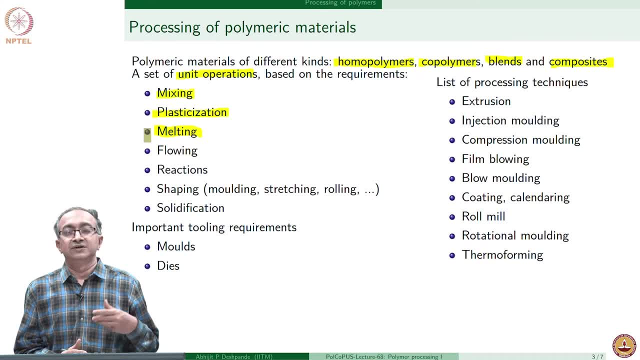 and rubber processing. again, temperature will have to be maintained from the point of view of maintaining the flow behavior as well as carrying out a reaction, because higher the temperature, higher will be the rate of reaction. So temperature is always a variable of interest during processing operations, either from a melting point of view or from a reactions point of view. So, of course, when you have process, Write O of A, don't waste any energy on it. So it will be entertaining in the context that we can do a lot of heavy work. So if allow me to question that, this is unique and what is the process? Where does 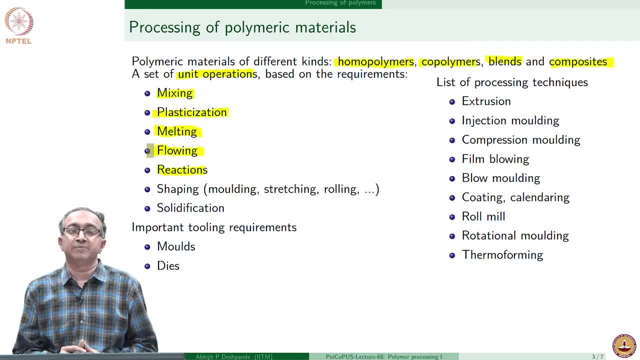 Of course, weather melting and reactions are happening. we will always have flow involved And so pumping actions, pressure generation, pulling and pushing operations, rolling operations, so all of these ensure that material gets pushed, material gets pumped and flow happens. And then we will have to make sure that the plasticized, flowing, reacting polymeric material 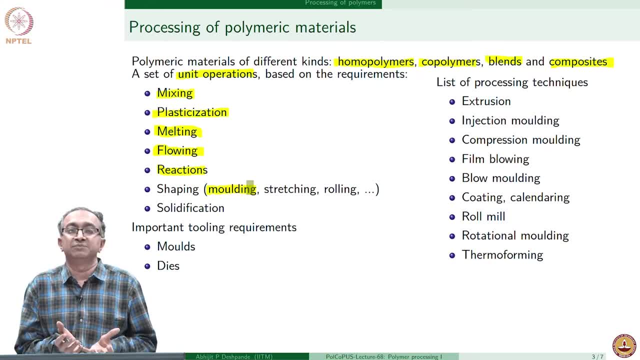 gets shaped by either enclosing the material in a mold or, if it is free flowing like a film, then stretching it to get a thinner and thinner film so that we get the final thickness that we want, or roll it so that again we can manipulate. So generally we have these processes. 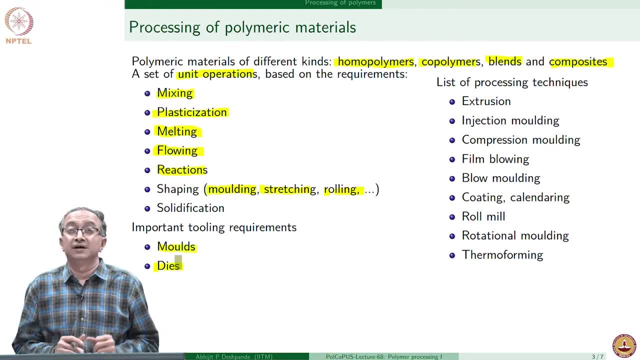 The tools which are called molds or dyes. molds basically encase the overall polymeric material, while dye is an opening through which the material is passed. So you can recognize immediately. for making fiber, a dye will be involved, because the polymer melt or a polymer solution will have to be pushed through an opening and then a 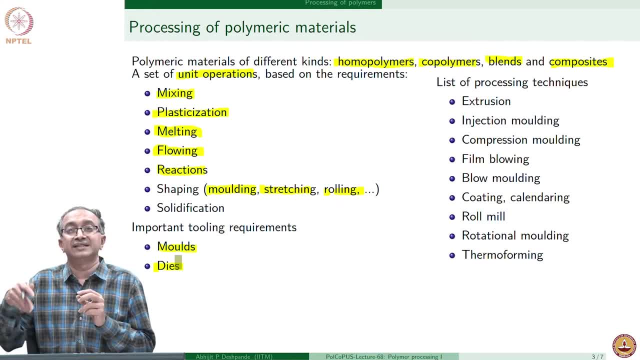 cylindrical jet of fluid will come out and that can be then stretched and we can operate to obtain the fiber of a given diameter. And of course the final stage is vitrification, solidification, crystallization, So all of the processes by which we will get the final state of the polymer. 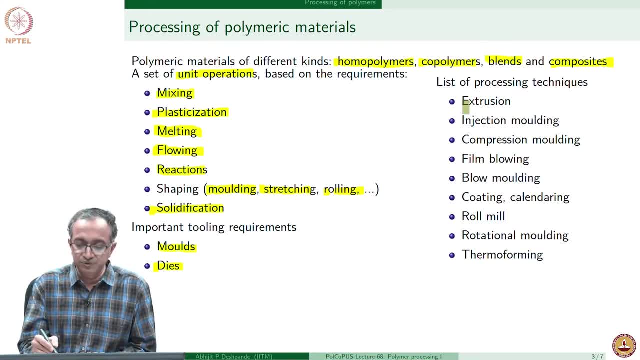 And so this is the overall set of operations. Extrusion is a very common processing technique where we do mixing, we also do compounding and also the shaping in terms of using dyes. So this is the overall set of operations. Extrusion is a very common processing technique where we do mixing, we also do compounding and also the shaping in terms of using dyes. 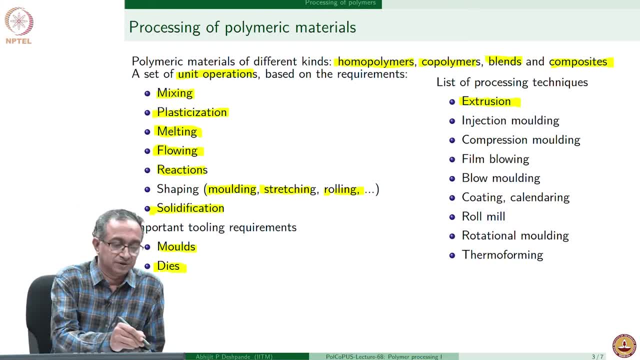 So this is the overall set of operations. Extrusion is a very common processing technique where we do mixing, we also do compounding and also the shaping in terms of using dyes. So some common term that you will hear is in terms of an extrusion dye. 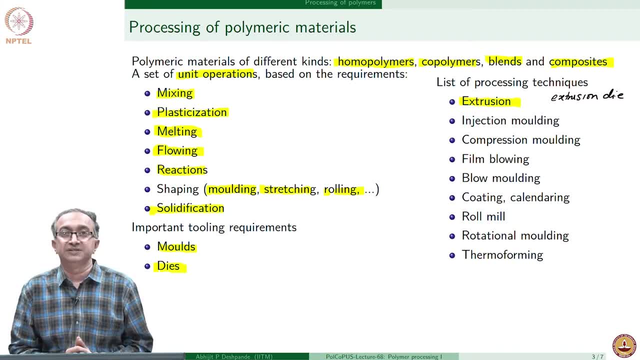 So extrusion can be used for both mixing and shaping operations simultaneously. So even wire coating, for example, when wire which is metal, let us say copper, on that we have polymer insulation. So this is also done through a wire coating operation which involves extrusion, in which 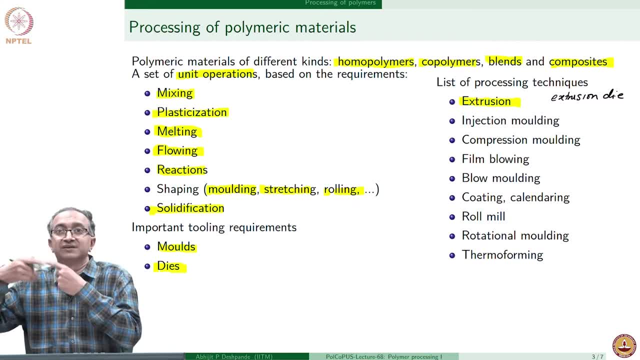 the wire itself is pulled and the polymer then can flow on the top of it. So what we have basically is a wire, thin wire, which is being pulled, And on top of that, because of extrusion, we have basically the polymer material. 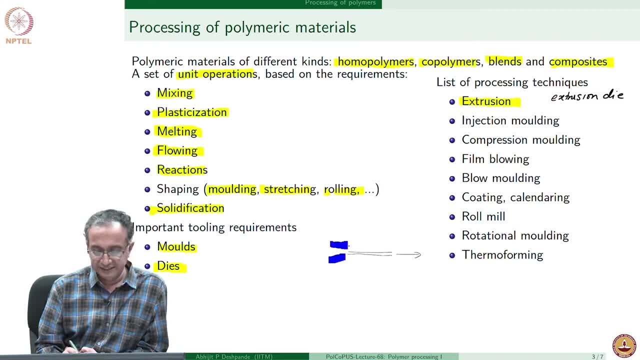 And this polymer material basically starts thinning out And then eventually we get a small fine coating. So the rate of pulling of this fiber, the wire itself, will determine how much polymer is getting deposited. Of course the rate of pumping of the polymer also determines it. 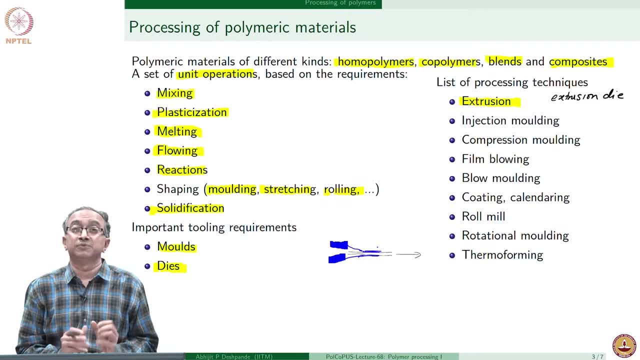 So you can see that if you want to analyze the polymer processing operation and come up with a control where you decide what will be the final thickness of insulation that you want, you will have to understand the flow behavior of polymeric system. Injection molding is the workhorse as far as polymers are concerned. because of its time, 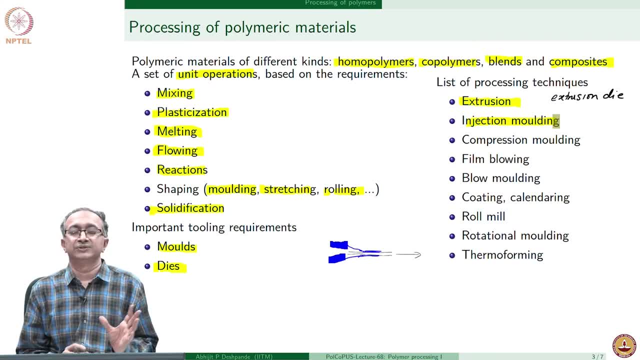 You can make an injection molded part in one second. So whether it is toys or whether it is fabricated parts in automotives sector, all of the places, household objects, we have lots and lots of injection molded products. The molds can be of very complex shape. 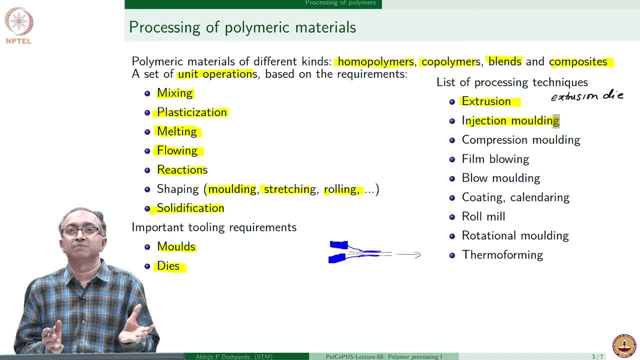 And in a single shot we can generate a very complex shape. And in a single shot we can generate a very complex shape. And in a single shot we can generate a product which is very complex in shape, but very quickly. Compression molding is a technique which is slower and it is used for largely flat or 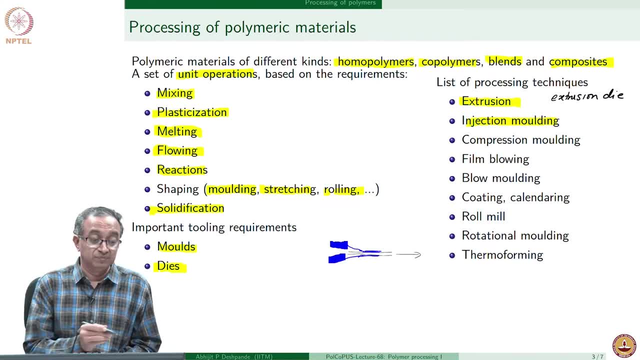 somewhat less complicated shapes. Film blowing again is a big operation, And that is based on the amount of films that are around us And in fact so. this also is a major reason for us to talk about single use plastics and sustainability, Because it is an operation. 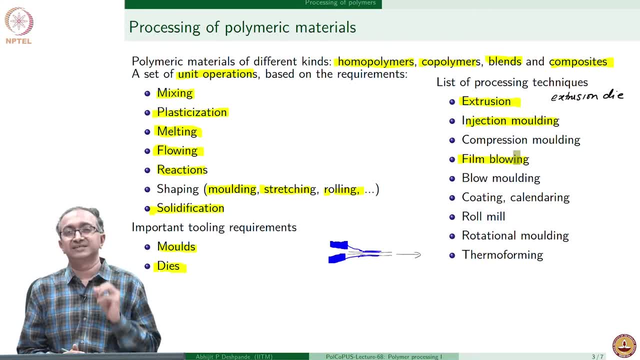 It is an operation. It is an operation in which you can produce films at an extremely rapid rate And the film properties can be controlled very precisely, Because we can control the processing, operation and flow, And what we will see is the extensional flow behavior of polymeric material so well that 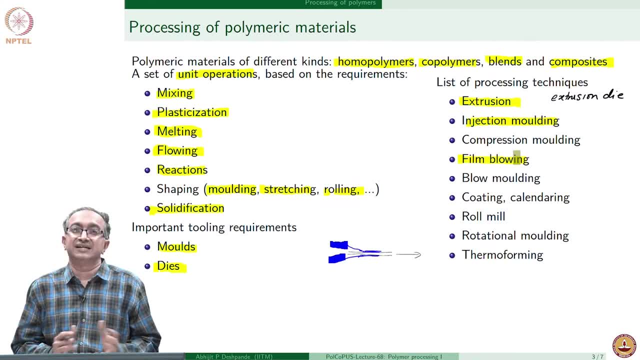 we can get these films at very large quantities with excellently controlled properties And therefore they are very inexpensive and they can be used in single use, where it is very easy to use and throw kind of applications, And so that is. we will look at that during extensional flow. 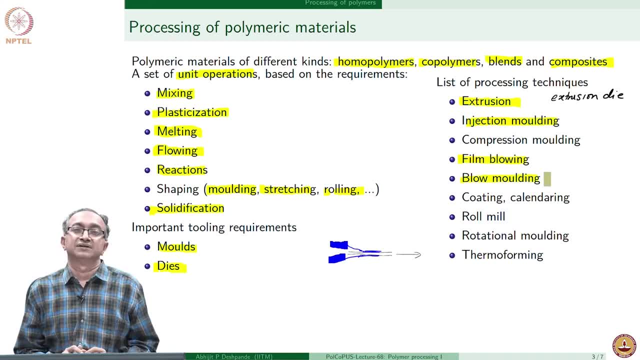 Blow molding is again a very popular technique where bottles, shapes such as bottles, are So, as the name suggests. so you can see that many of these are suggesting the way in which it is carried out. also, So, injection molding: there is an injector which is used in case of blow molding. blowing. 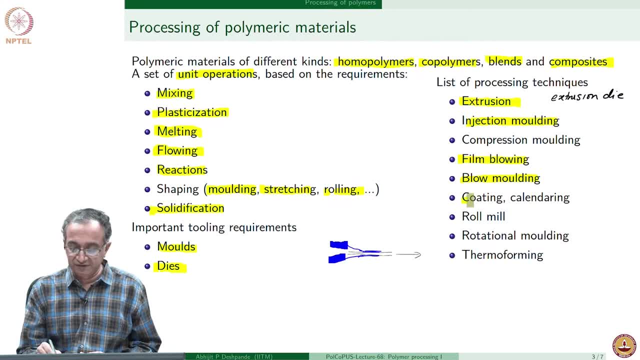 is happening, along with the mold, Of course, Coating and calendaring operations, which involve a set of rollers on which fluid- polymeric fluid- is coated or calendared onto a set of substrate. Roll mills are used in rubber processing for so this does the role of mixing as well as. 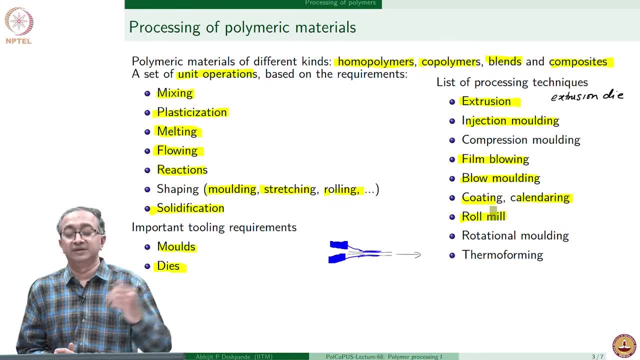 shaping the rubber before it can be finally made into the part. Rotational molding is a very common technique to make tanks. Especially in India we see the water tanks for overhead storage And most of them are made using this rotational molding as a technique. 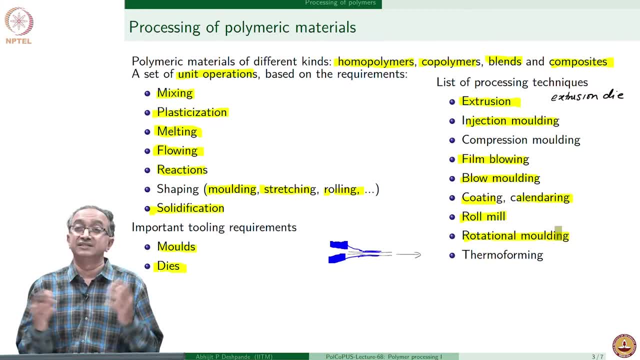 Again, it is a technique with, in reasonable amount of time, you can make these cylindrical tanks. And thermoforming is similar in some sense to compression molding, But thermoforming is an idea borrowed from metallic processing, where we can take a sheet and then just do a quick stamping of it and shape it, while compression molding involves 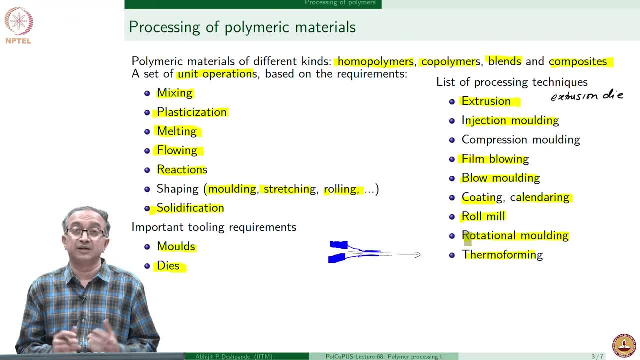 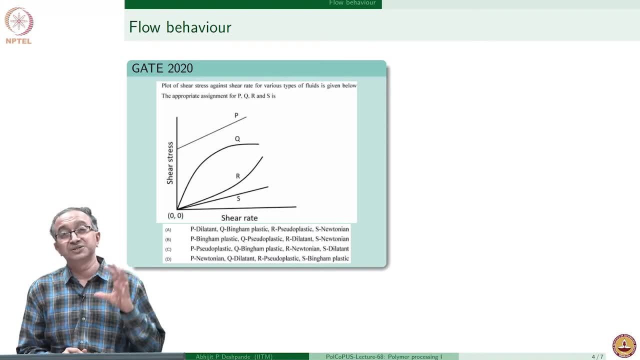 quite often reactions, and therefore it takes more amount of time. Well So, thermoforming is quicker. So this is a broad survey of these polymeric processing techniques, And in each of them polymer is flowing. It could be a pre-polymer, it could be a resin, it could be a final polymer, it could be with. 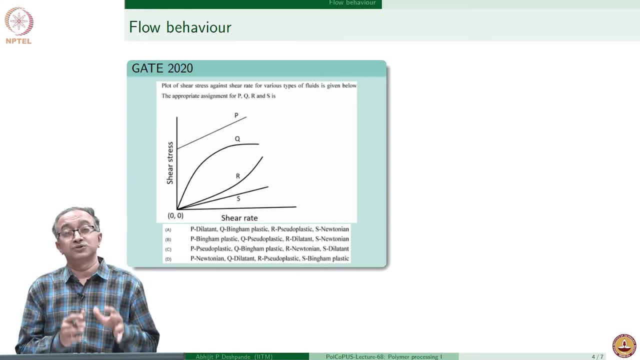 different additives, such as plasticizer. it could also be with fillers and fibers. So therefore, the flow behavior of polymeric systems is extremely important, And this is highlighted in this question here Where. So the way to look at the flow behavior is to look at what happens to the material when. 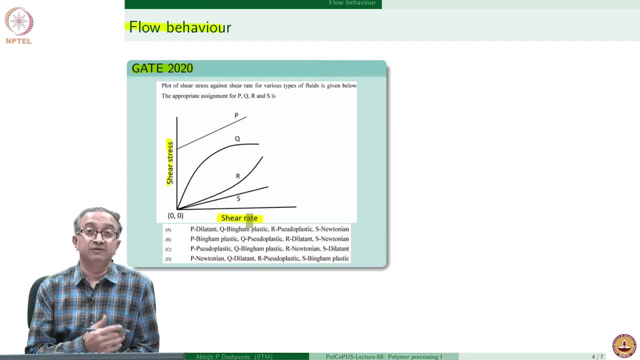 we apply a rate on it and we wait for the steady state. So this is basically data where it is called steady and it is also called shear steady- shear Steady- because we apply a stress, wait for shear rate to become constant and then measure. 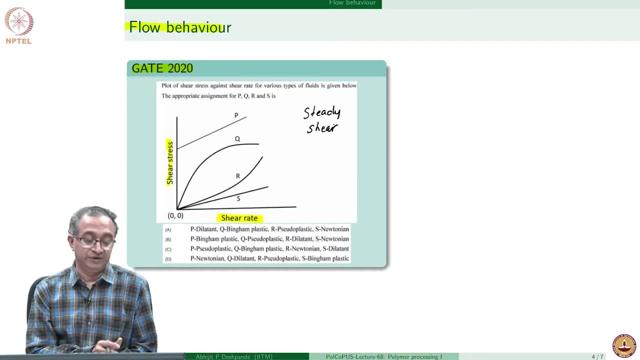 both stress and rate, or we apply a constant strain rate, wait for stress to reach steady value So we can measure both stress and strain rate, And then we can plot. And so for a Newtonian fluid we know that stress is proportional to shear rate. 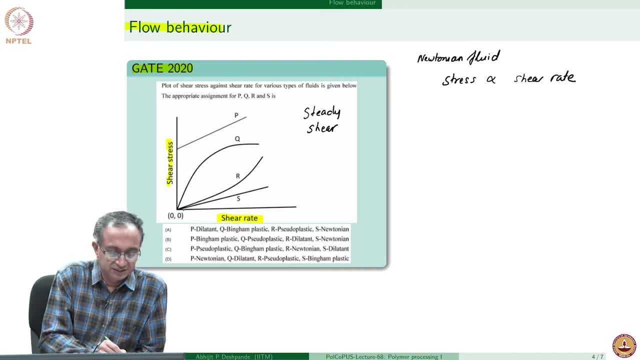 And, of course, the proportionality constant is viscosity. So this graph here is basically for Newtonian fluid. Okay, Okay, Okay, Okay, Okay, Okay, any polymer processing discussion, these kind of graphs where we have different types of fluids like dilatant, bingham plastic, pseudo plastic, and so can you just spend some time. 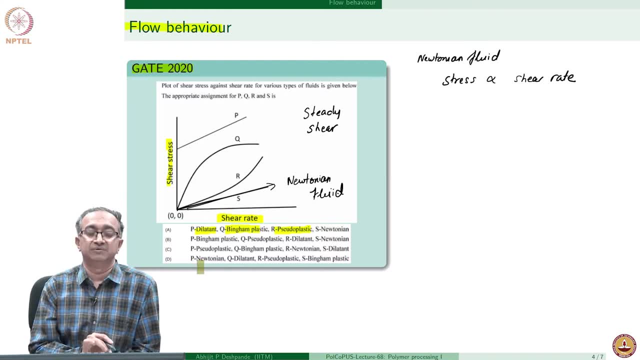 and try to think of what is the meaning of each of these term and why do these graph signify? and the reason for doing so is flow. behavior will depend on how is material responding to stress, and each and every processing operation involves different amount of shear rate. 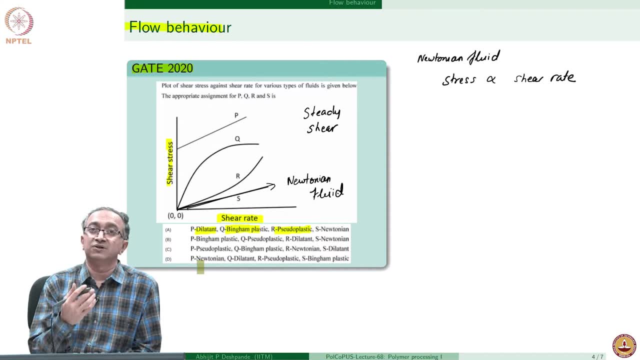 Injection molding involves very high shear rates. compression molding involves less shear rate, So therefore the same polymeric material may behave one way in injection molding will behave completely differently in case of compression molding because the stress in the material is not directly proportional to shear rate, like Newtonian fluid. 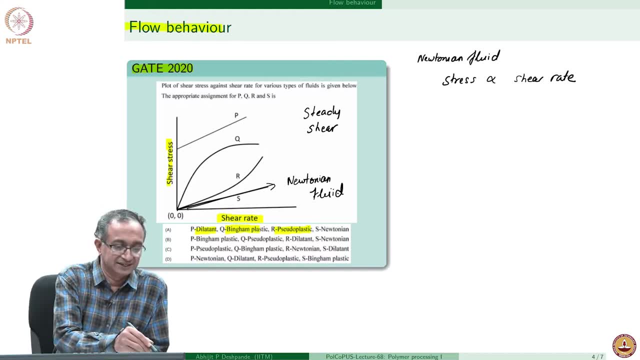 It is a complicated function. You can see that in some cases There is an increase, some cases there is a decrease, some case there is a direct jump. So each of these shows very different behavior and we need to characterize this, if we have. 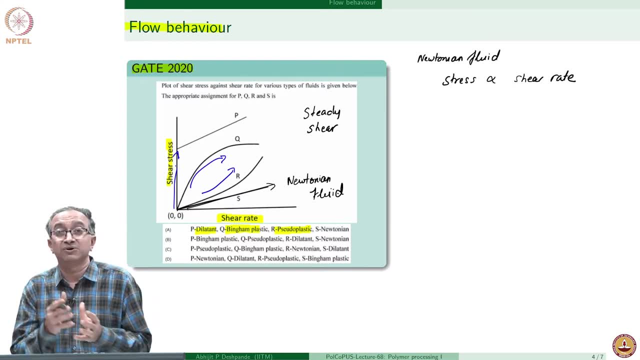 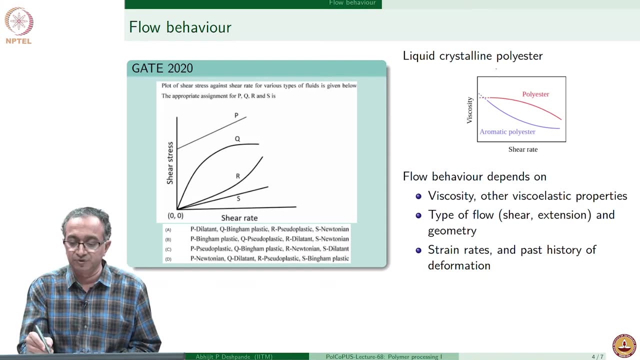 to study flow behavior of a polymeric system in the context of polymer processing. This is just to highlight also that even if you talk of the same family of polymers- in this case let us say polyester- But if you have the polyester in the form of a polyester, 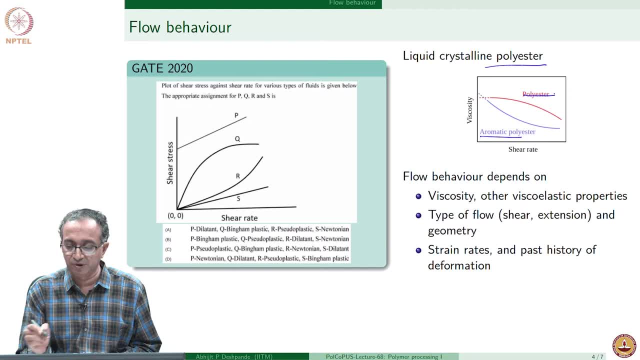 Polyester, Polyester, Polyester, And the form of a liquid crystalline polymer or the normal polyester, which is a flexible macromolecule. the viscosity versus shear rate can be very different for the two cases, And what I also want you to think of is how to go back and forth between these two graphs. 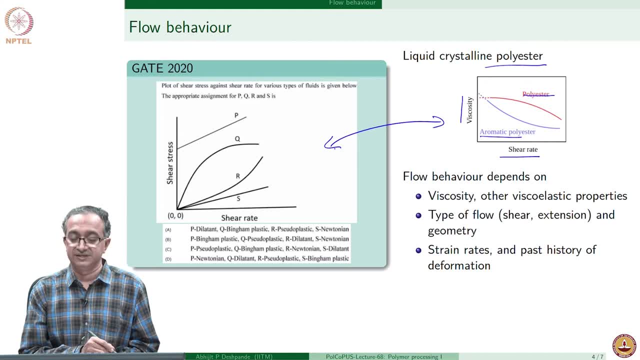 Stress versus rate, and the other case, viscosity versus rate. And of course, we define viscosity as stress divided by shear. Just look at them. Yes, So if you were to plot the red data on this graph, how would it look like? 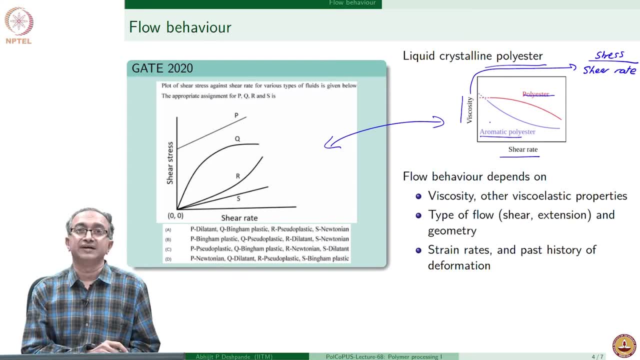 Or if you were to plot the blue data on this graph, how does it look like? And so there is a significant difference, especially in terms of low shear rate behavior. For the blue, the aromatic or liquid crystalline polymer, it appears that viscosity increases. 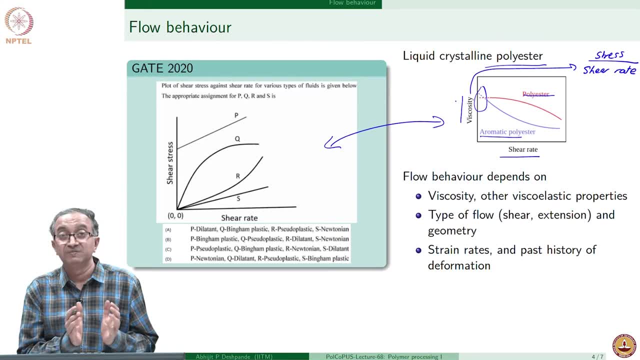 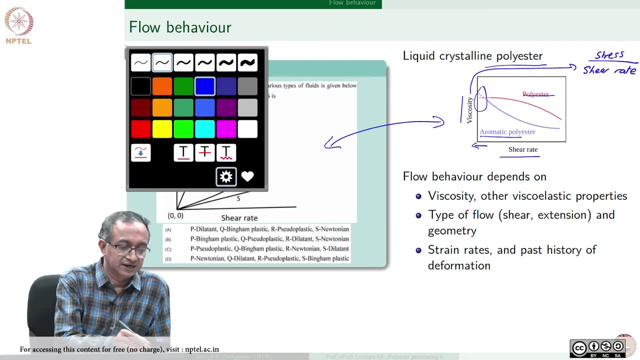 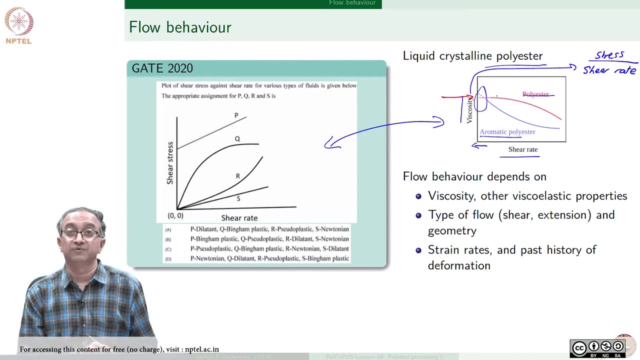 and continues to increase and may even go to infinity when we go to lower and lower shear rate, While the polyester, the viscosity at low shear rate seems to become constant. So this is a constant value of viscosity for polyester. So very different behavior and wherever there are low shear rates, this can be very crucial. 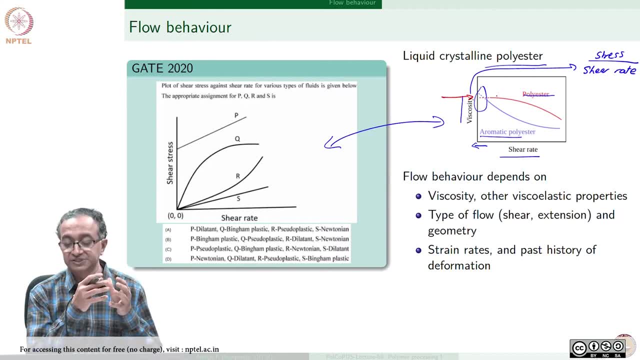 So liquid crystalline polymer, wherever shear rate is very low, viscosity will be extremely high, velocities there can become very low and we can have a stagnation, While in case of polyester, viscosity will not go beyond a certain upper limit. So you can see that if we have to analyze the polymer processing operation, avoid a 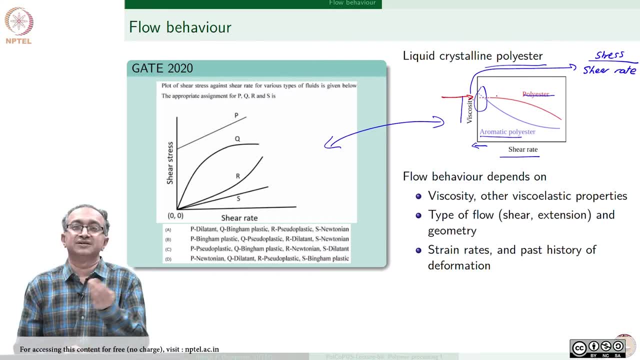 stagnant place, because stagnant place implies that polymer will just circulate there and it is not really moving. And in a processing operation we make the material flow and fill into a cavity, mold, or we will pass it through a die. So our objective is to have all of the polymeric material move or flow. 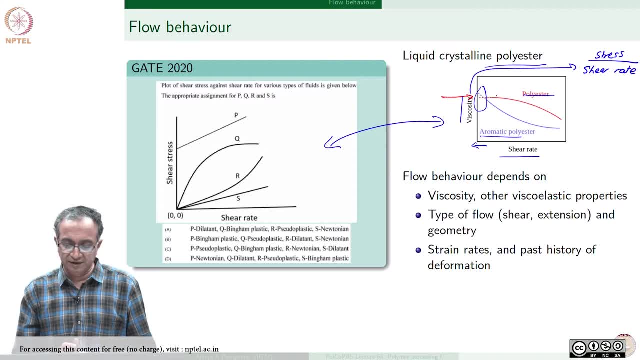 And so, generally speaking, this is the case. So this is the case. So this is the case. So, generally, to analyze the overall response, the flow behavior depends on viscosity. However, that is not the complete picture, because polymeric materials have a certain 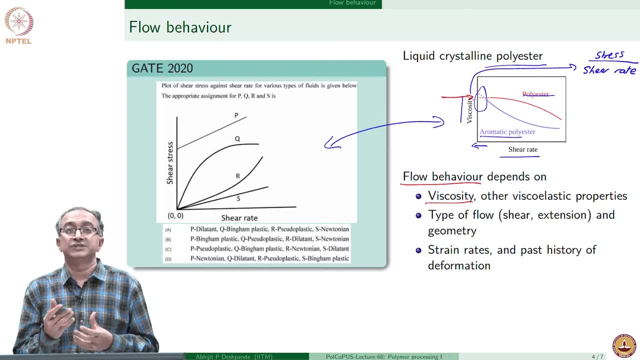 elasticity. We have these segments which can stretch and recover. Stretching and recovering is nothing but elasticity. So therefore, even in a molten state, even when pre-polymer is there and molecular weight or molar mass may not be very high, the segments have a tendency to stretch and recoil stretch. 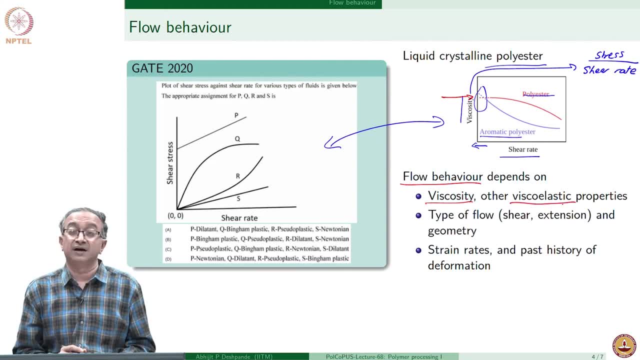 and come back And therefore polymers are, in the fluid state, quite elastic and therefore they are viscoelastic materials. It also depends strongly on what type of flow and what is the geometry of flow, because polymeric fluids given the ability to stretch and recoil, 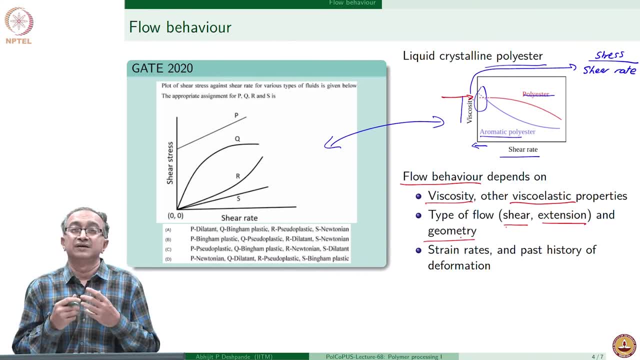 They exhibit very different behavior if they have been going through a very gradually changing geometry or a sudden contraction or a sudden change in geometry, because what happens is polymer, on average, has a certain conformation. As soon as you change the geometry it has, it is possible that it can acquire other conformation. 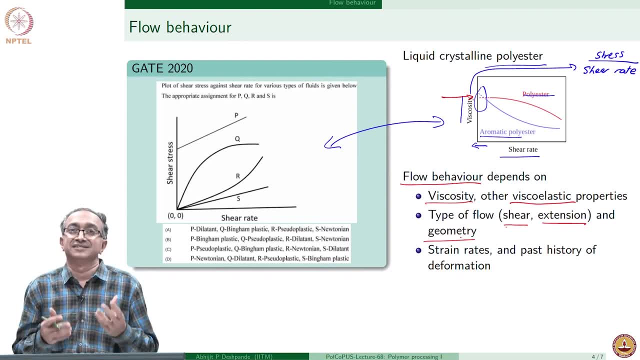 And the going back and forth between these conformation is elasticity. So therefore how this happens determines the overall flow behavior of polymeric materials. So generally, strain rate, past history of deformation, all of these influence the current state in the material. 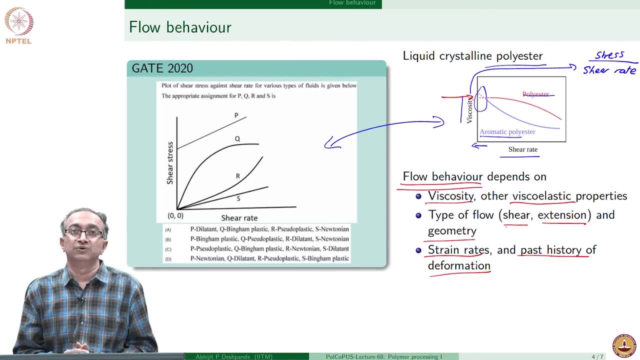 And this is what we saw during viscoelastic models also, we saw that, whether it is Maxwell model or standard linear solid model, its current state of stress determines on past history of deformation that the material has undergone, or other way to say, it is the current. 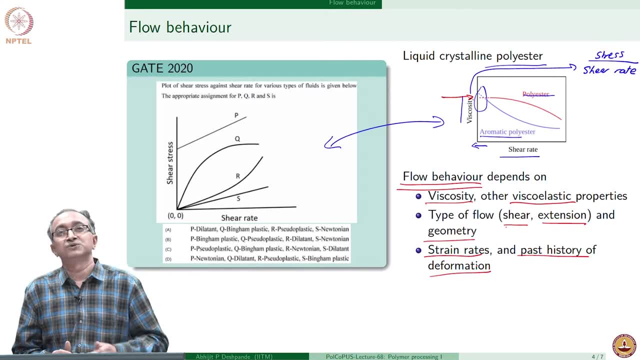 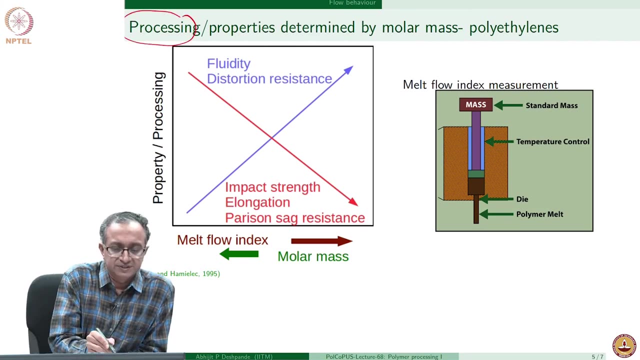 state of stress depends on not just current values of strain, strain and strain rates, but it may depend on stress rate and variety of other rate quantities. So generally this is of great interest because processing determines the properties And all of this is influenced based on molar mass. 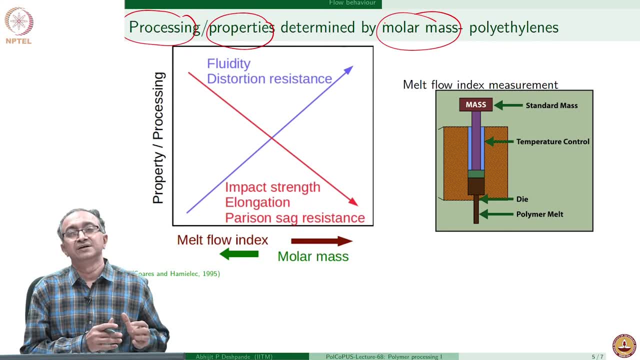 So when we want a certain property, We may require, may require a certain molar mass, but if you want ease of processing, we may require another molar mass. So, for example, the fluidity or the distortion resistance of the material increases whenever. 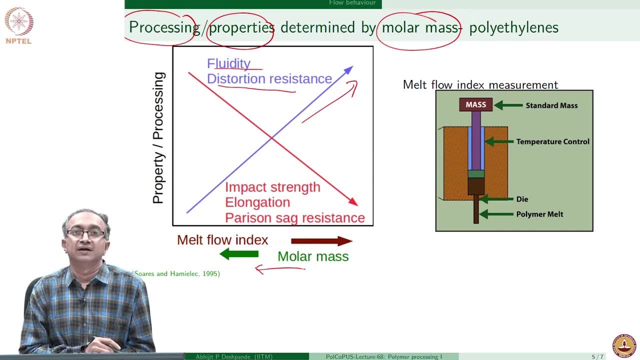 molar mass is decreasing. When molar mass is low, it is easy for the polymer to flow. However, many of the properties of the polymers will go down if the molar mass is lower. So there is some optimum always. 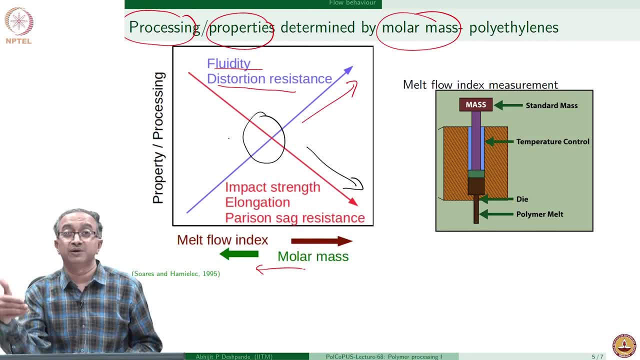 So, whenever we think in terms of development of a polymeric product, so far in our discussion we have only talked about properties and how properties can be optimized- how properties can be maximized. But the success of polymer product will also depend on whether we can make the polymer. 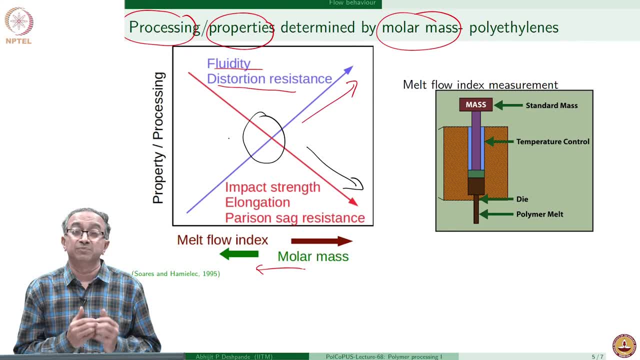 product And, in other words, can we process it, And so processing may require a different set of properties, or, as scientists and engineer, we will have to then think of new ways of processing so that we can achieve the desired product. So therefore, in general, the processing structure properties that we discussed have 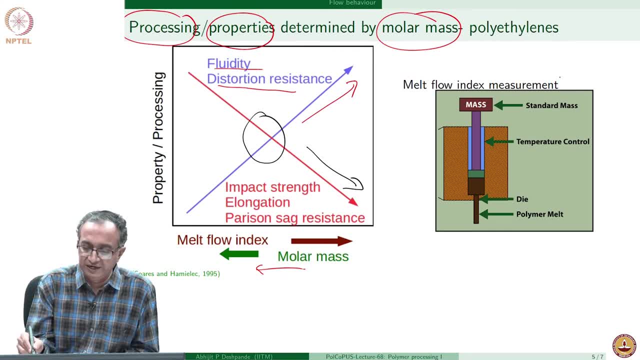 to be taken together. One industrial way of measuring the flowability is called med flow index. This is a simple technique in which we apply a mass on polymer melt And this is so. there is a basically piston which is pushing the melt And, given standard mass, we just measure what is the amount of melt that comes out in a 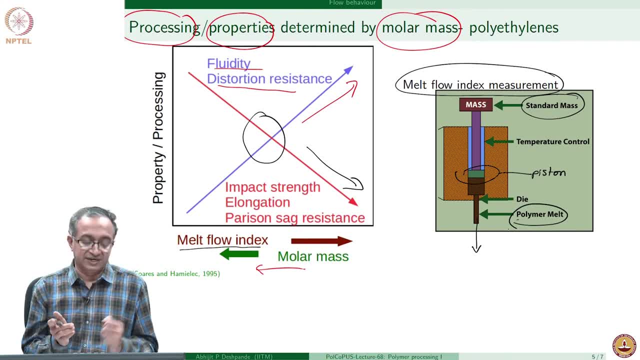 given amount of time, And so this is a very standard way. It is a very simple method In which, if you look at the industrial grades of polymers, MFI will be mentioned, And this is inversely related to viscosity. I hope you can see why I am saying that. 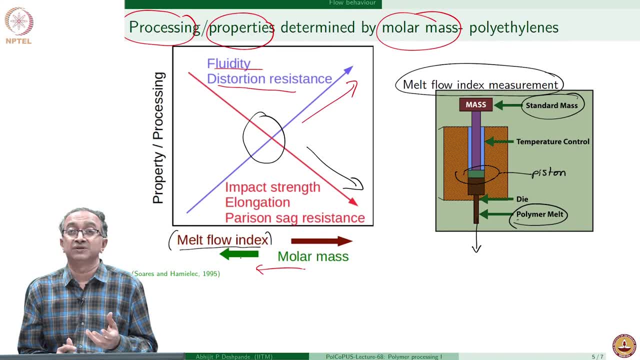 Because at a given mass, if more amount of polymer comes out, melt flow index is higher. But since more amount of polymer is coming out, it implies that viscosity is lower. That is why flow rate is high and more amount of polymer comes out. 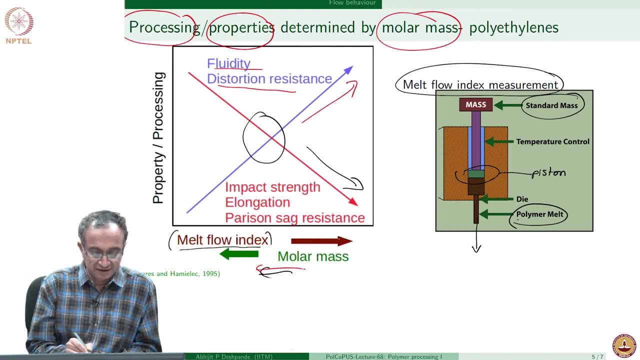 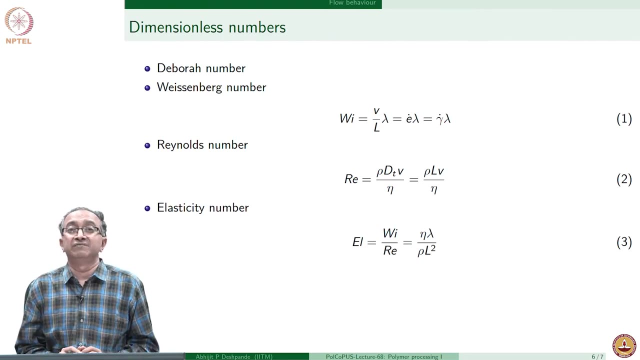 So that is why molar mass And the And the melt flow index are inversely related to each other. When molar mass increases, the melt flow index will be lower, And so the. when we are looking at all this flow behavior and different characteristics, 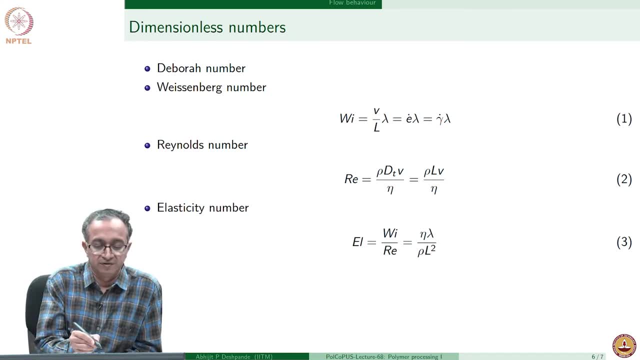 what are the dimensionless groupings which are of importance? Of course, Deborah number, which talks about the experimental time scale and the material time scale. We have discussed this several times, So this is important Specifically for flow. we also have the Weissenberg number, which is based on the 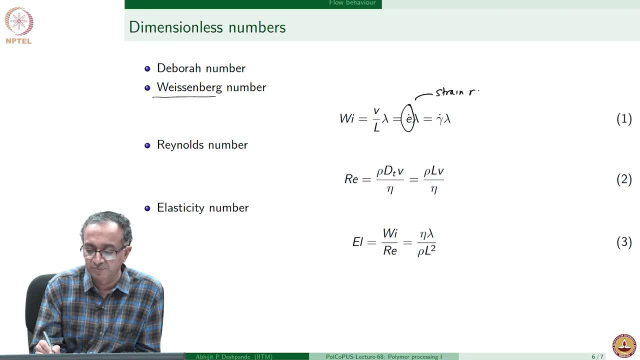 strain rate of the polymer processing operation. Because in polymer processing we will definitely be flowing the polymeric material And, for example, if we have a screw and a barrel in case of an extruder, the screw is pushing the polymer And so the velocity next to screw will be very high. 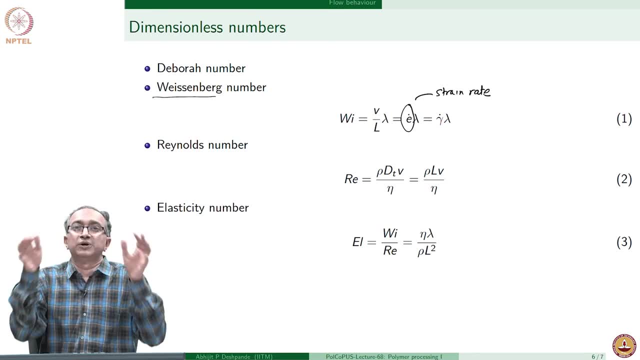 But outer barrel And the velocity of the polymer will be 0 because the barrel is stationary. So then the strain rate determines the rate at which the pushing is happening, And so that time scale associated with strain rate and the time scale associated with material 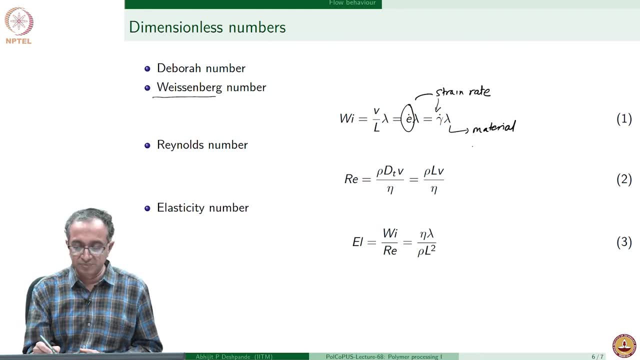 decides what will be the behavior. Reynolds number is, of course, the comparison of the inertial to the viscous forces in the material. the ratio of Weissenberg number and Reynolds number can also give us another way to look at how much is the elasticity in the polymeric materials.